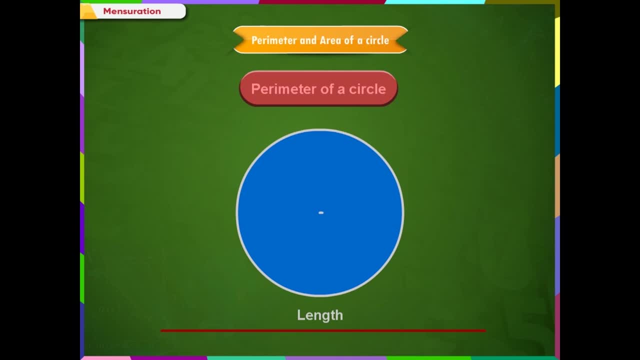 we will get the measure of the circumference, But it is difficult to do so when the circle becomes larger and larger. Hence we use the formula to find the circumference of a circle. Formula for the circumference of a circle is Pi into diameter, or Pi into 2R or 2PiR. 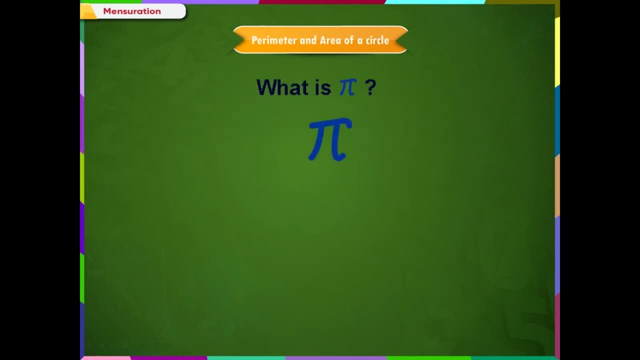 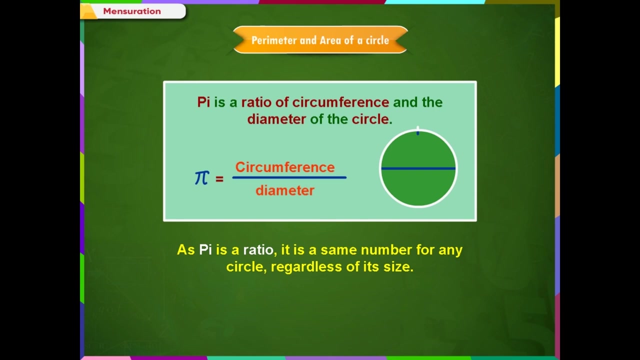 What is Pi? Pi is a Greek letter and is spelt as Pi, which is a special number. Pi is a ratio of circumference and the diameter of the circle. Hence, Pi is equal to circumference divided by diameter. As Pi is a ratio, it is a same number for any circle, regardless of its size. 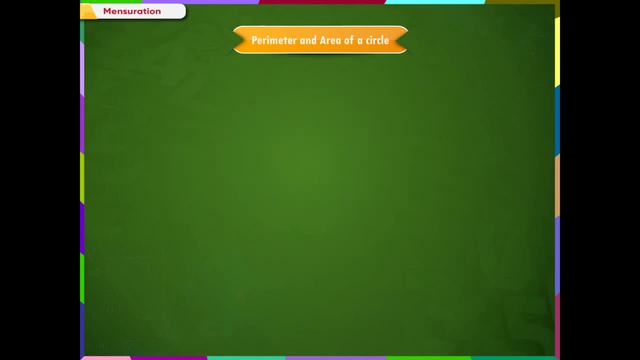 To understand how Pi is related to circle, let us consider two circles of different diameters. Let us assume that the diameter is flexible and we can wrap the diameter along the edge of the circle. If we start wrapping them around the circle, three diameters is also not enough to cover the whole circle. 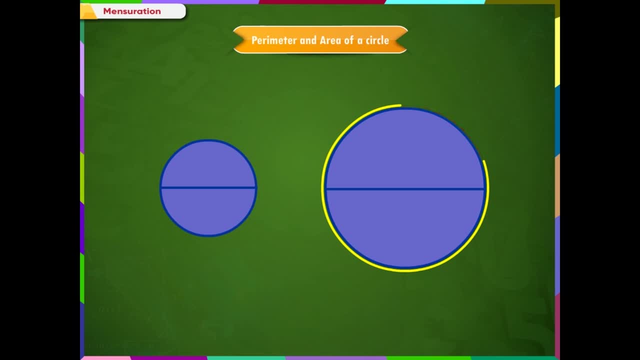 Observe the figure, A small space is left. This small space is approximately 0.14 of the diameter. Therefore, we need 3 diameters and 0.14 of the diameter to cover the circumference of a circle, whether big or small. 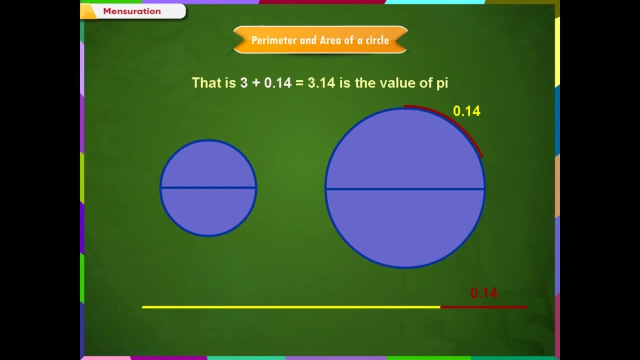 That is, 3 plus 0.14 is equal to 3.14.. Therefore, 0.14 is the value of pi. 3.14 diameter is equal to 1 circumference. Therefore, value of pi is equal to 3.14.. 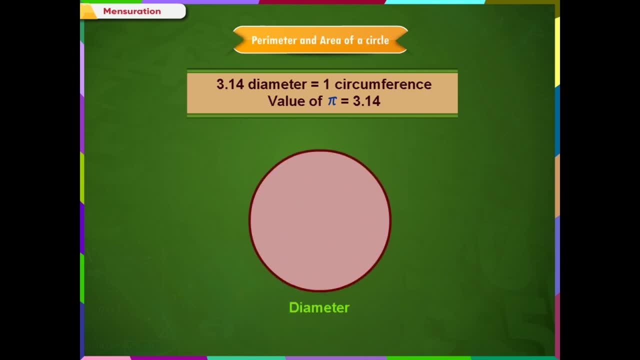 Therefore we can say that if we know the diameter or the radius of a circle, we can find the circumference of the circle. Area of a circle, The measure of the region enclosed inside the circle, is called its area. In the figure shown, the coloured part inside the circle is the area of the circle. 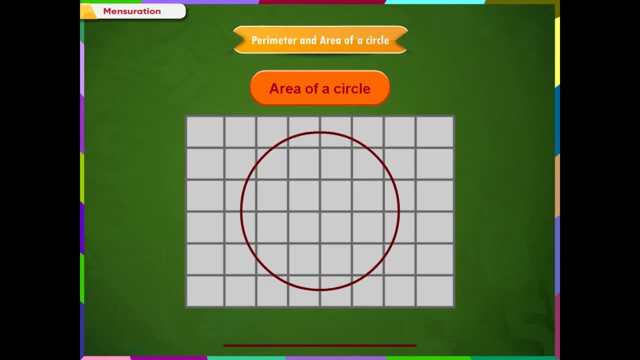 If we place the circle on a grid paper and count the number of squares on the grid, we can get the area of the circle in square units. Observe the figure shown on the screen. If each square is 1 centimetre, then the area of the circle is 16 square centimetre approximately. 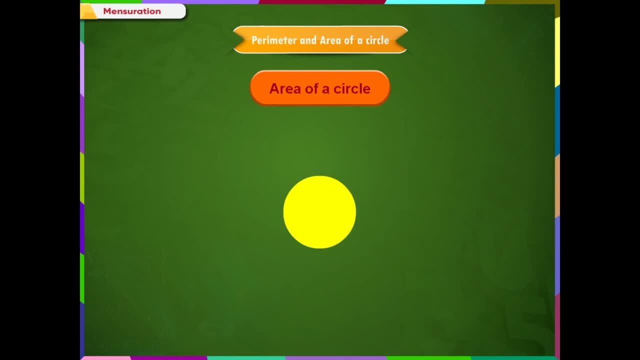 But this method is difficult to calculate when the area of the circle becomes larger and larger. Hence we use the formula to find the area of a circle. Area of a circle A is equal to pi- r- r square, where r is the radius. Let us understand from where the formula for area of circle has come. 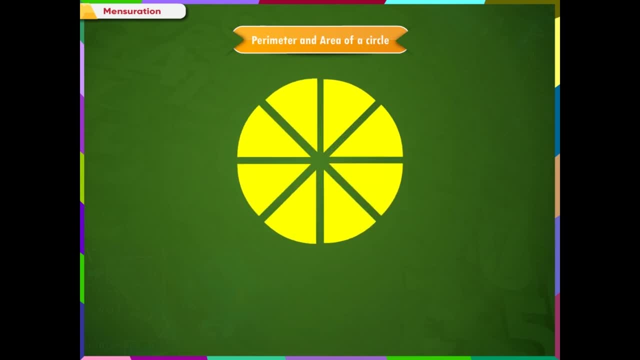 Take a circle and cut it into 8 equal pieces like this, and arrange them into a rectangular formation like this. As you can see, it hardly resembles a rectangle. Next, we will divide the circle into small pieces. We divide the circle into smaller equal pieces and arrange them into a rectangular formation. 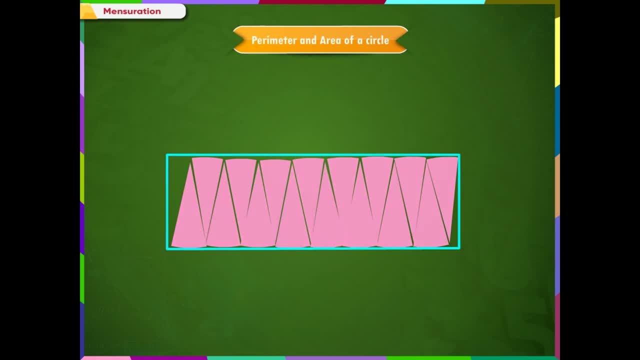 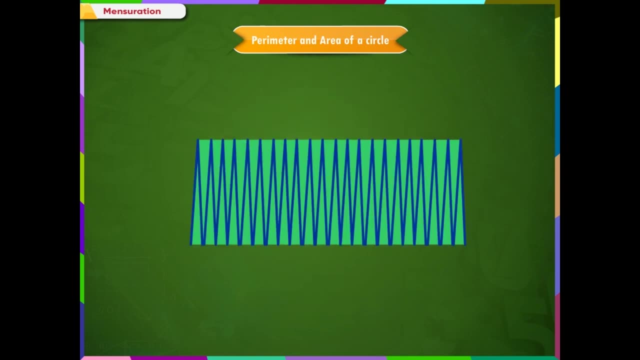 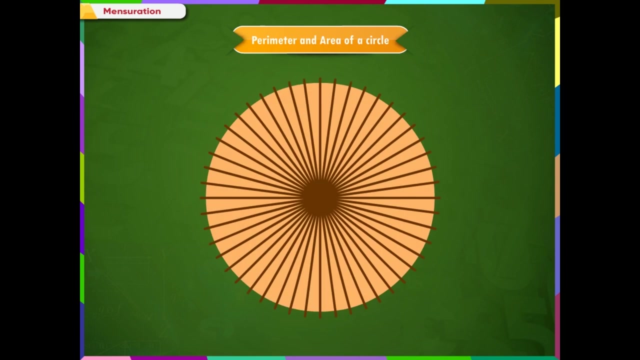 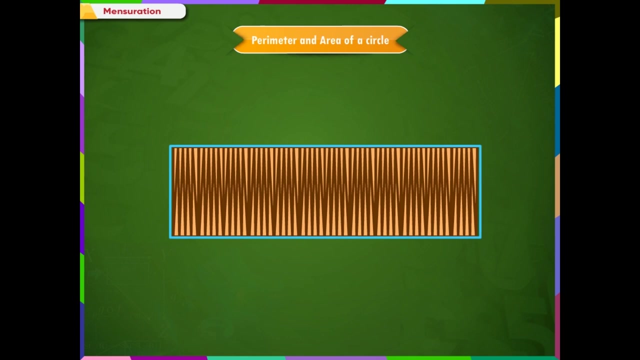 We still see that it doesn't resemble a rectangle. Now if we divide the circle into smaller, equal pieces and arrange them, we see that it is closer to a rectangle. So how small we divide the circle into equal parts to get a figure almost closer to or equal to a rectangle. 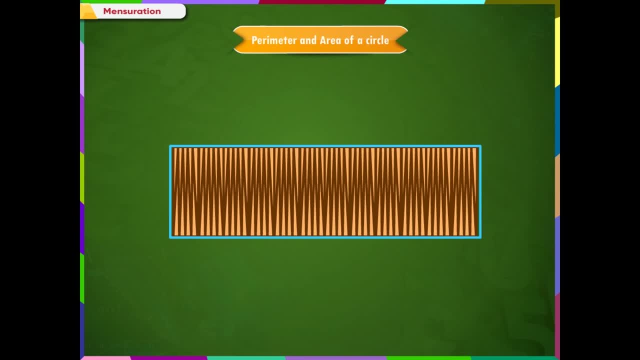 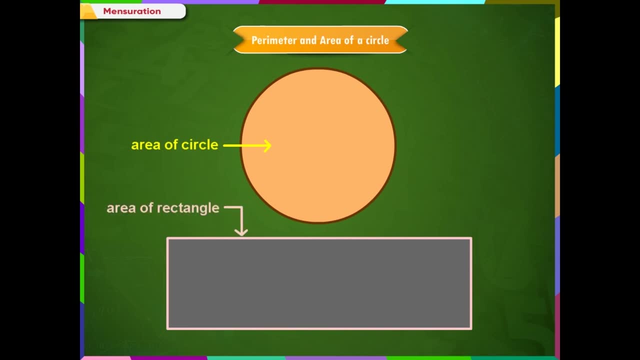 we divide the circle infinitely many times this way to get a rectangle. So area of the circle is equal to area of rectangle, which is equal to length multiplied by breadth. The breadth of the rectangle, as you can see, is equal to the radius of the circle. 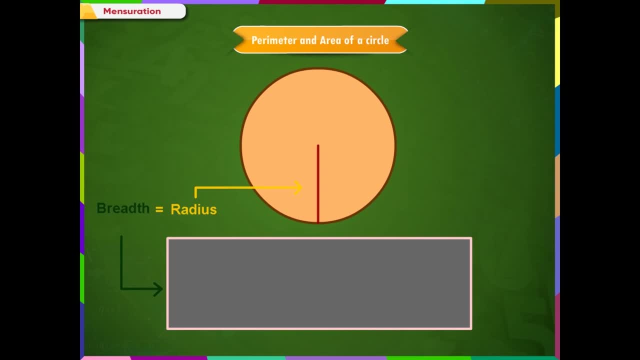 So breadth is equal to radius. To find the length we need to look at the circumference of the circle And when we compare the length with the circumference we see that the length is half of circumference of the circle. We know that the circumference is given as 2 pi r.